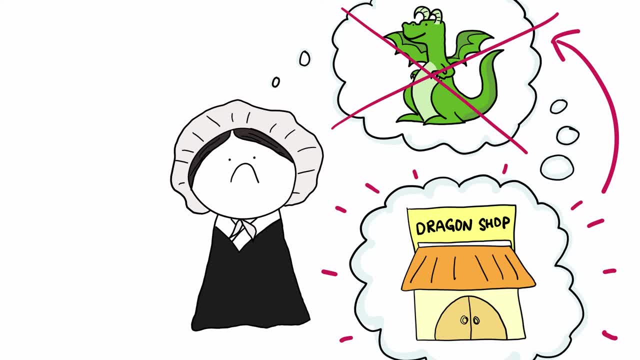 So as much as Mary or I or you want a pet dragon, we can never have a pet dragon. And because her having a pet dragon reduces to the problem of finding a dragon shop, this means we can never find a dragon shop too, Because if we found a dragon shop we would have a pet dragon, Which 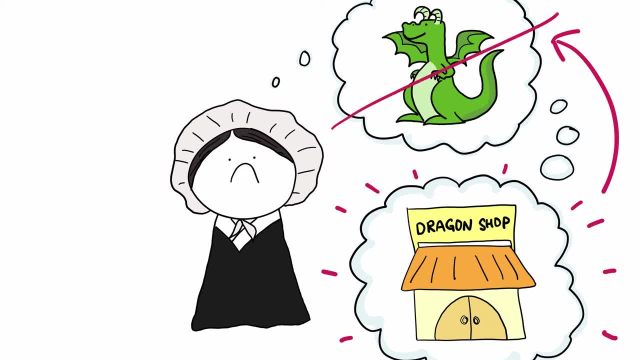 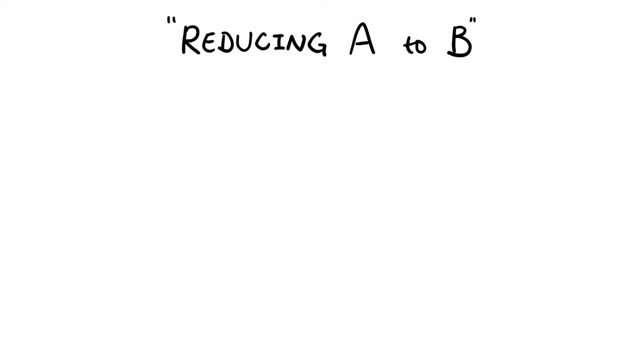 is a contradiction, since dragons don't actually exist, Despite the confusing terminology. reducing a problem to another problem does not mean one of the problems is smaller or necessarily easy. A reduction of problem A to problem B simply means that we are looking at A in a different form. 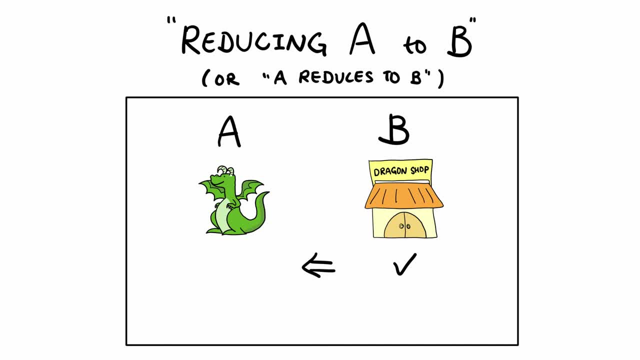 And if we solve problem B, we can solve problem A, And if we cannot solve problem A, then we most definitely cannot solve problem B. This part is important for using reductions to show that a problem is unsolvable, Or in terms of computer paper. 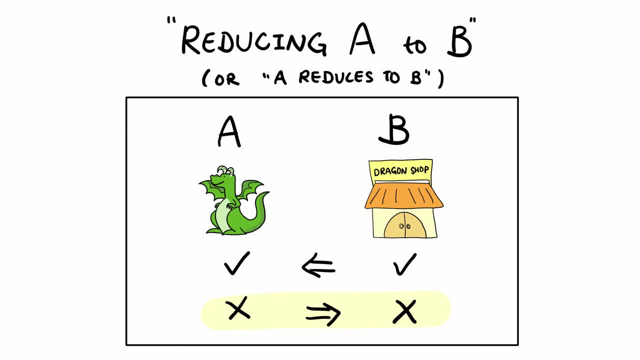 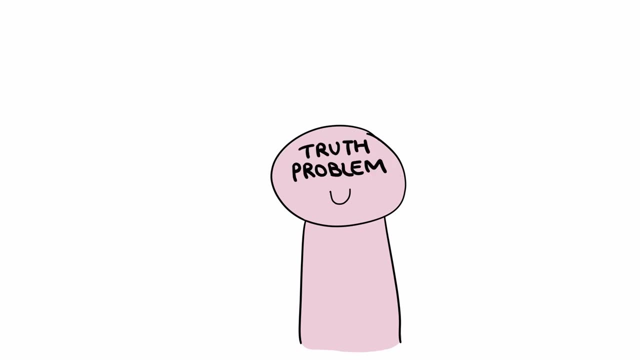 theory undecidable. We'll now look at an example of how we use reductions to show that a problem is undecidable. Let's say we want to show that this problem is undecidable. Let's call it the truth problem. The truth problem asks whether 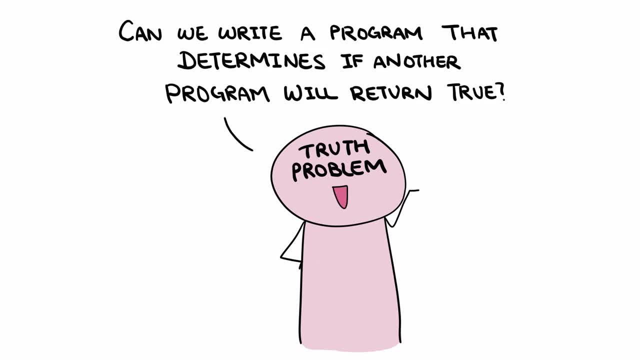 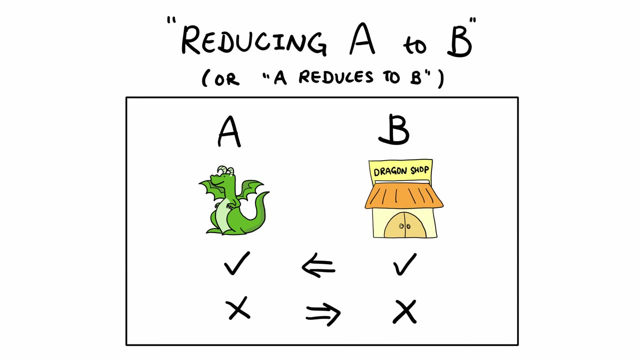 we can write a program that determines if another program will return. true, So how can we show that the truth problem is undecidable through a reduction? Now remember how we mentioned that if we can reduce problems A to B, and by knowing A is undecidable, then we show that B is undecidable. Well, since we want to show 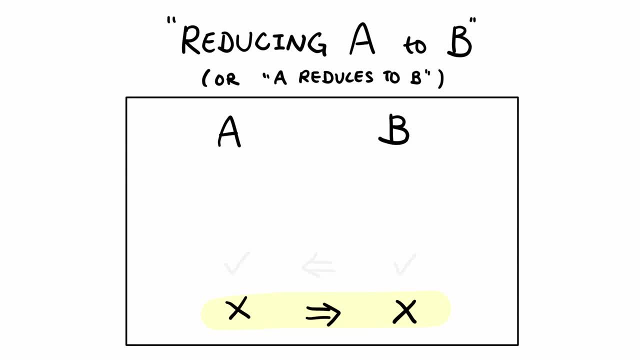 that the truth problem is undecidable. we'll have the truth problem be B and put some other problem that we know is undecidable to be A. In another video we saw that the halting problem was undecidable, So let's have the halting. 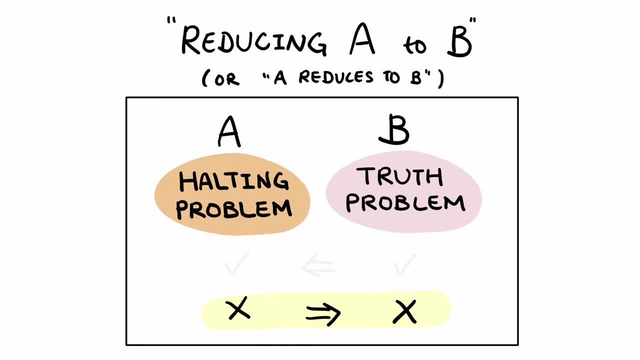 problem be A and, like the dragon and the dragon shop, showing that problem A reduces to problem B will mean that by solving B, we will solve A. However, similar to the fact that dragons cannot exist, the halting problem A is undecidable, which means the truth problem B that it reduces to must also.